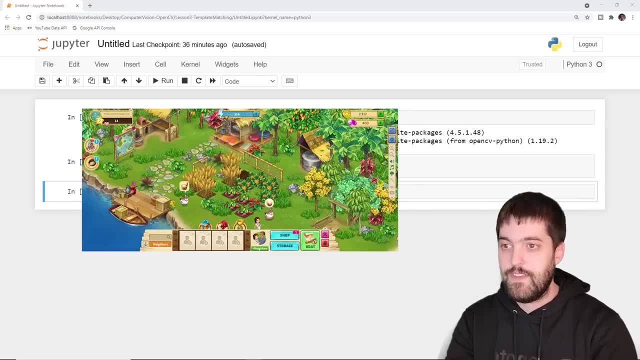 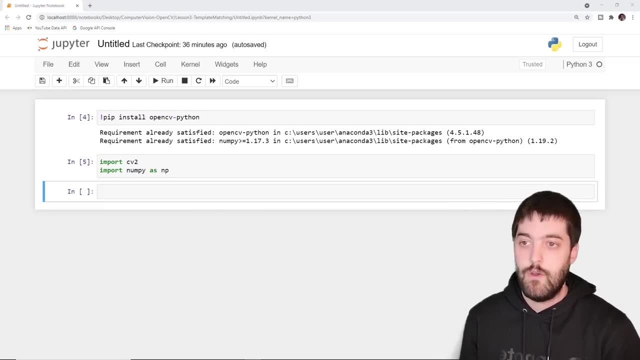 source image. Now you can imagine that as a live camera feed or some type of original image that you're looking for another object inside of. So you've probably seen ones where you detect a mask or you detect an eyeball or whatever it is out of the image. We're going to call these our farm image. 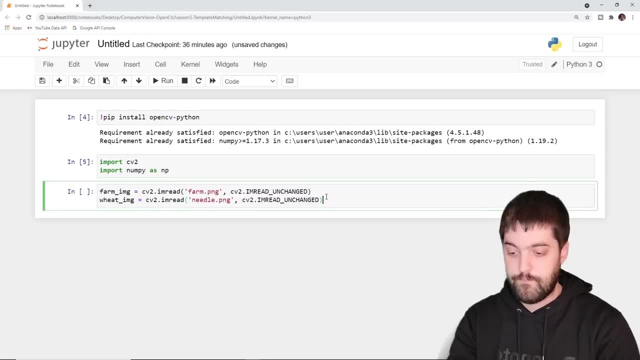 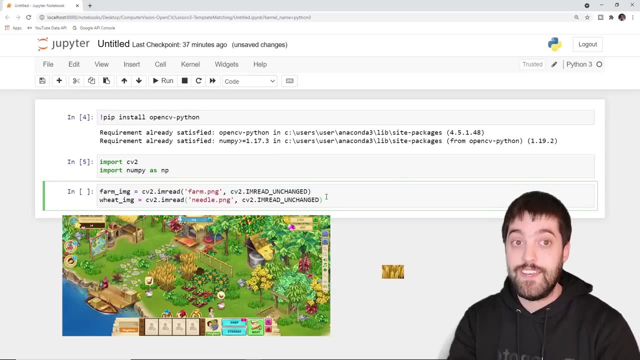 and our wheat image. So if you look at these images, it's just a simple game, like a farming game, and we're going to try and pick out the different instances of wheat inside that image. Now, this is a little tricky because some of the wheat images are covered up by other things and sometimes there may be different shades. 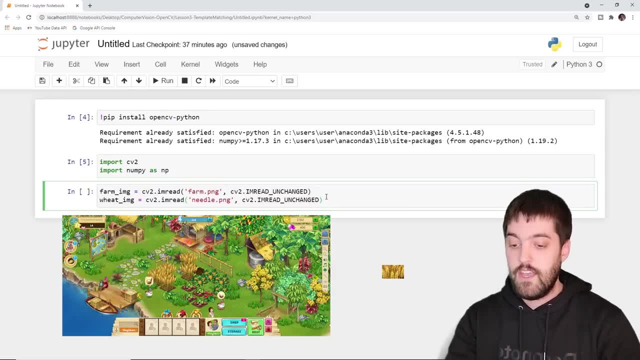 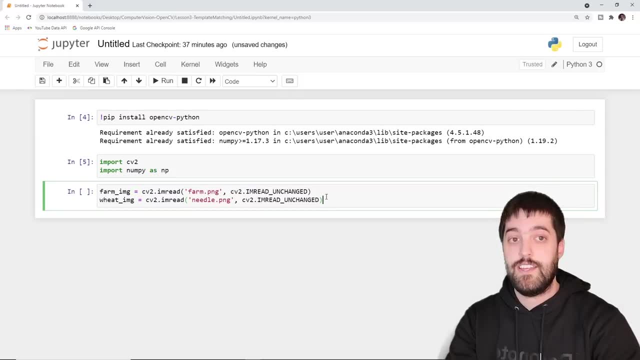 maybe the game turns from day to night or something like that, and you can imagine this in a real world setting as well. If you want this notebook, this code or these images, they're all in the GitHub in the lesson three folder, So you can grab them from the home page and you can see that they're. 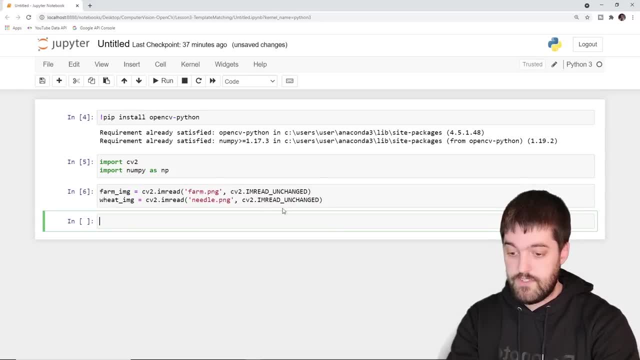 the description. We're going to run shift, enter and pull in our two images. Now these are in the same directory as the script, so you'll notice I'm just referencing the image, the file name, directly, and then to show these images, I'm going to create a couple more blocks of code here. This is going. 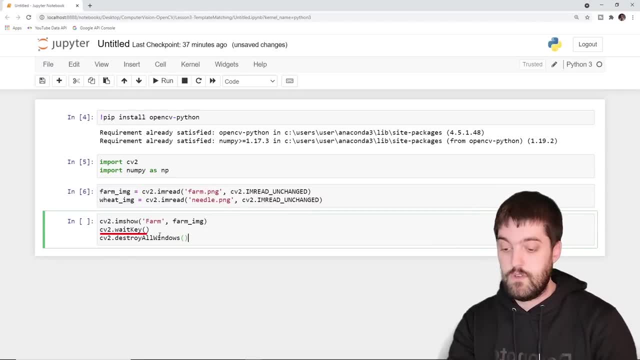 to be to show our farm image. You can see that we do cv2 wait key. Now that's going to allow it to stay up until we hit a key and then destroy all windows. This is something that I have to do in Jupyter Notebooks so it doesn't freeze the notebook. So if we do shift enter, here you can. 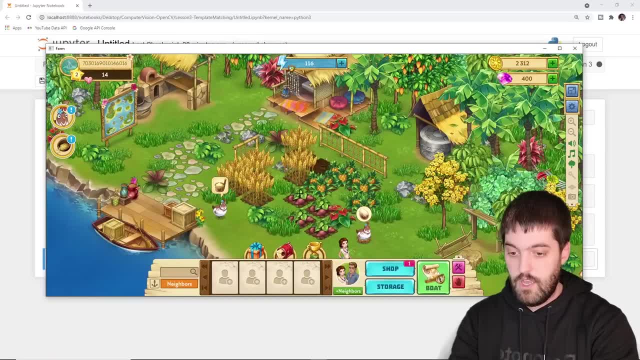 see it appears just to hang, but if you look down in your taskbar, you should now have an image pulled up and you can see that this is going to be our original image and we're going to try and detect wheat images out of it. So now what I've done is I've created a needle image. what a play on needle. 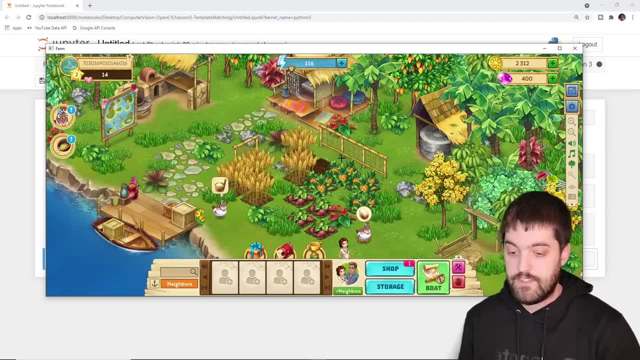 in the haystack. So we're going to look for an image inside of this image. Now, what I did was, straight out of this image, I created a needle image, So I'm going to look for an image inside paint. I just cut out the wheat image that we're going to look for Now. my hope is that we detect. 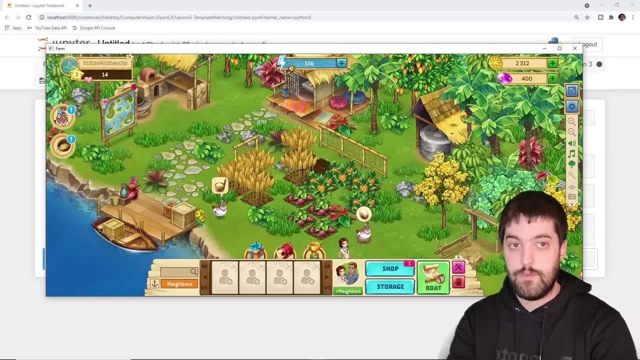 multiple instances of wheat, and then we can do something based on that information. Maybe, if it's like a security camera or something like that, we throw an alert. If it's something like you're creating an automated game or whatever it is, maybe you're clicking in that location. 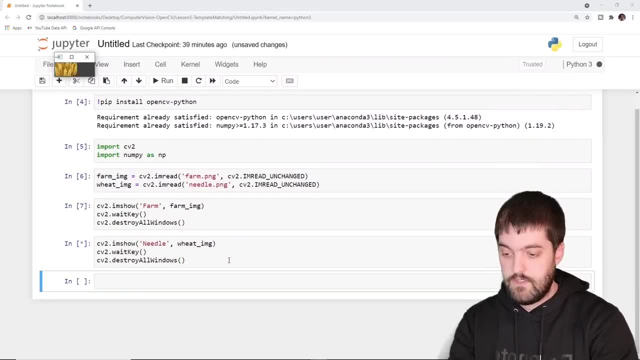 to harvest the wheat. Next, let's show our needle. So the needle in this case is this tiny image here. So we're going to cut out this image and we're going to look for an image inside paint. You can see, it is literally something that I cut out of our original farm image. So that's what. 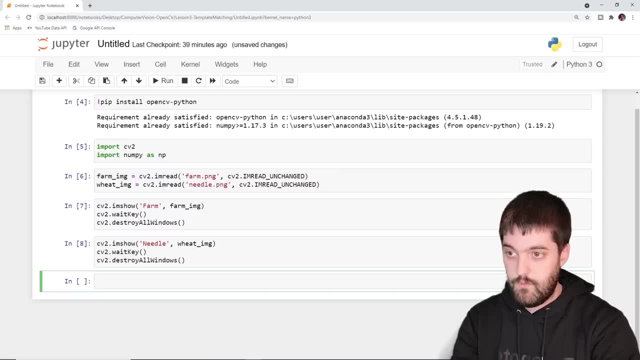 we're going to be looking for. We'll close that as well, and we'll reference these back a couple times when we're going through this demonstration. Now for template matching. what we're going to do is we're going to use different algorithms that I'll show here to try and see a match in our 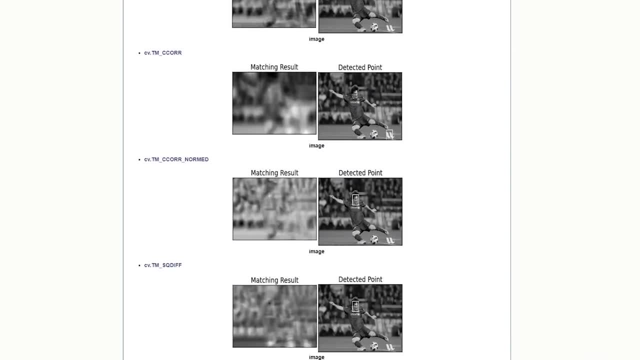 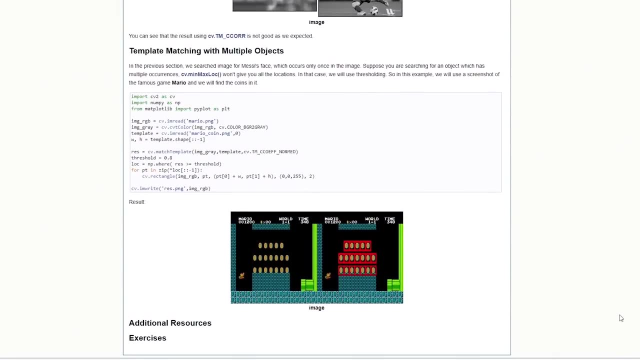 image. So we're going to try and pull out features in a match. Now I'll note the docs here and you can read up on each template. So I'm going to go to template matching and I'm going to go to different type of method and there's a lot of mathematics that goes along with it. But 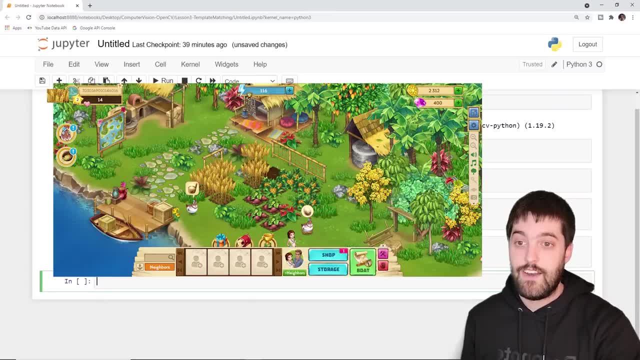 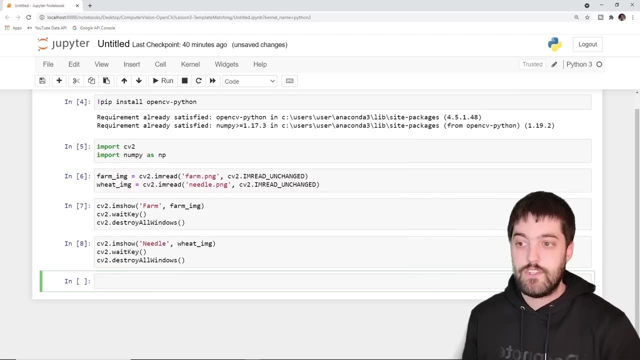 essentially, what we're going to do is slide our needle image across our original image and try to find a match. Now, for each of those locations that we test, we're going to get a value back. that's how close of a match it is. So what you're going to see is, when we originally do this, you'll 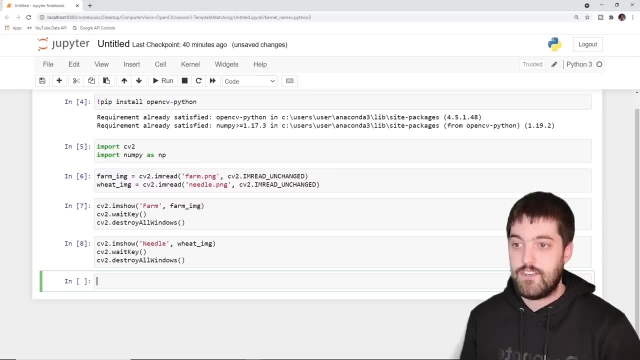 see almost like a heat map that shows where the best matches are. So let's go ahead and take a look at what that looks like here. So what we can do is we can choose one of the six template matching algorithms to use, and then we can run it and get our result. So what I'm doing here is I'm 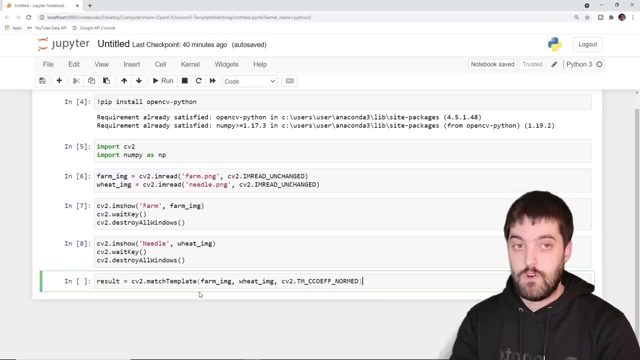 doing cv2.matchTemplate. I'm doing the image that we're looking for, the needle inside of which is our farm underscore image, and then our needle image itself. So this is what I'm looking for, which is the wheat image. We can run this, and I've also picked one of the algorithms that I'm going to. 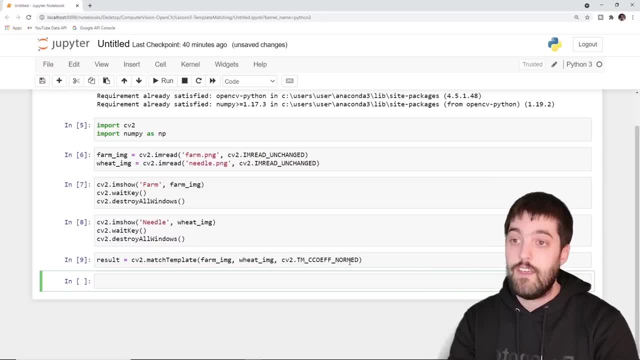 use. You can use whatever one you would like. If you're doing this in a real world project, I would suggest testing them all and seeing what works best in your case. Now, this is pretty cool. we can actually grab that result and show it to the screen, just like our other items. So what I'm 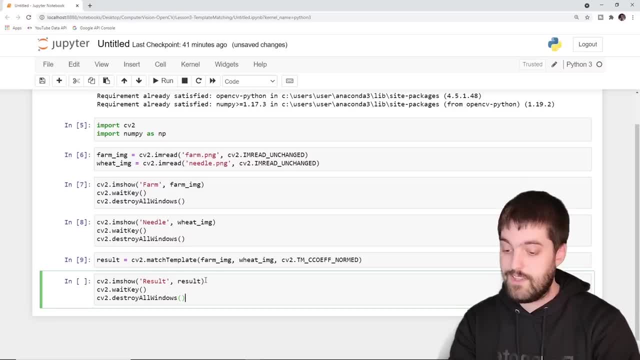 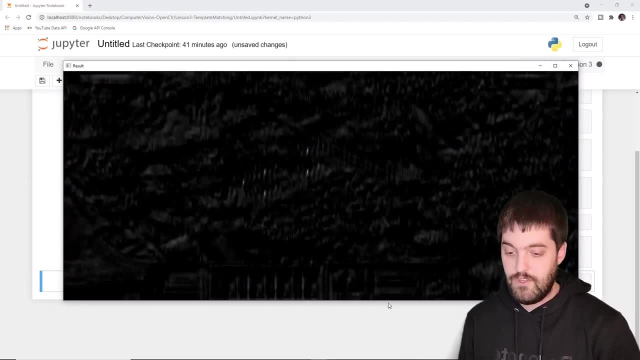 going to do here is I'm going to do imshow again. with our result? the same exact weight key destroy all windows and if we look at this you'll see. at first it doesn't look very useful. but if you look at this image you'll notice it's a black and white image and there's some white markings along it. 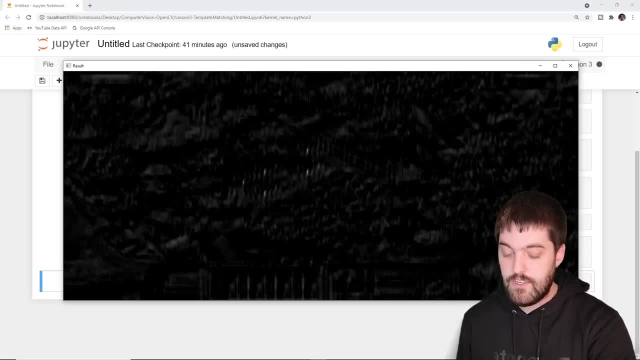 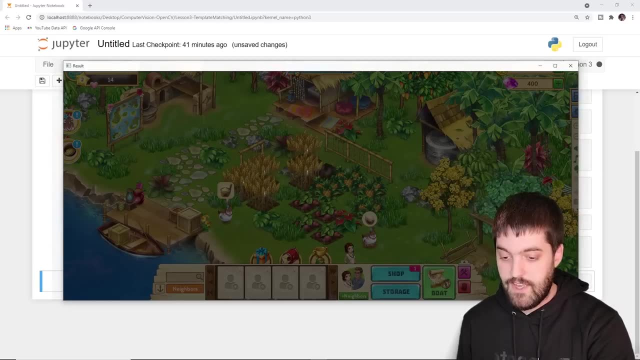 You can tell where it's lighter and where it's darker. So these light images are where there's a closer match. Now, if you look closely and overlay our original image here, you can see that it picks out five pretty distinct white points. Now those white points are where the wheat is. So we know we. 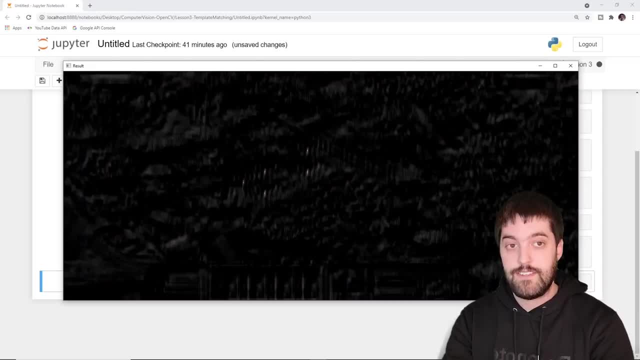 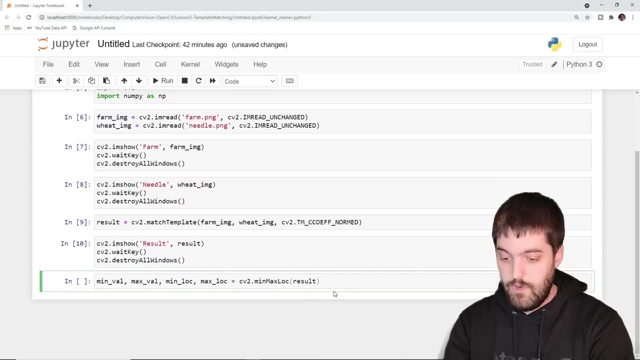 have something going here. This is a pretty good. it's finding some pretty good results right now. So if we want to get our best matches back, we can use cv2.minmaxlocation on our result. So what this is going to do, it's going to return four things. It's going to return the minimum value. 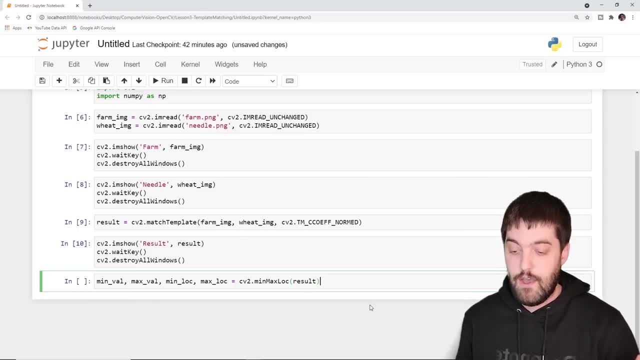 so that's the worst match of all the matches. The maximum value, which is the absolute best value of the best match. It's going to return the minlocation, so that's the location of the worst match and the max location, which is the location in the best match. So if we run this, we're going 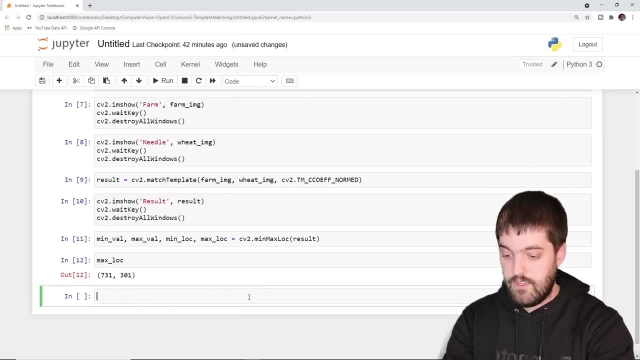 to get some values back, and one of those values is our max location. Now, this is very useful. this is the xy coordinate of our best match, So with that, we can draw a rectangle around our original image to highlight where our best match was. So let's go ahead and take a look at that. 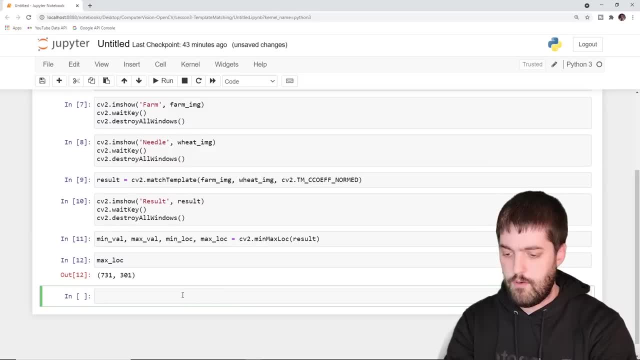 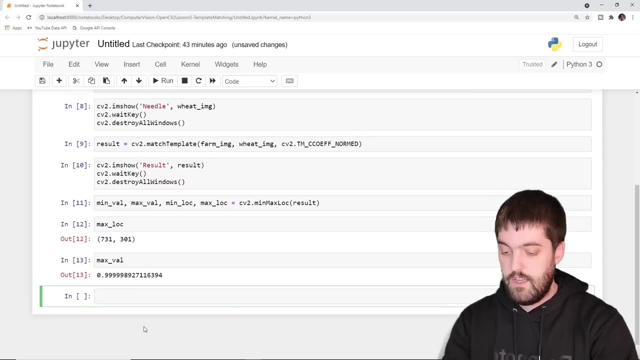 And actually, before we take a look at that, let's also look our max. This is our max location. Let's also take a look at our max value. Now you'll notice that our max value is a point nine, nine nine percent match, which. 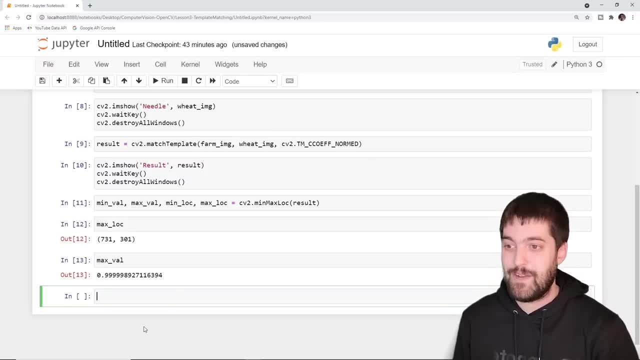 is really good right, Which makes perfect sense because I literally copied and pasted the image from it, So it should have a pretty good match. So we're gonna use that later. So we're gonna later we're gonna say a threshold of what is a. 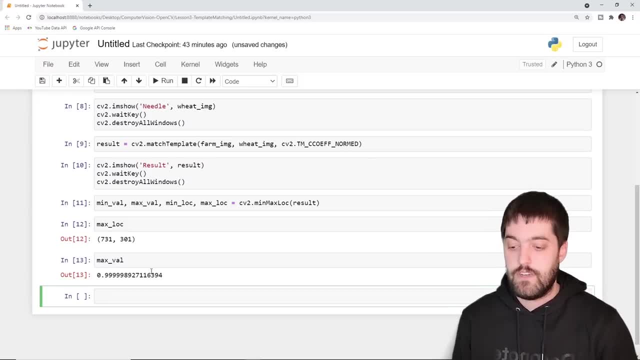 good enough match. So obviously in real-world examples you're not gonna get a nine, nine, nine, nine percent match very often. So what is a good enough match that we still think it's wheat? That's what we're looking for here. So with our best match we're not quite to the multiple matches yet. Let's try. 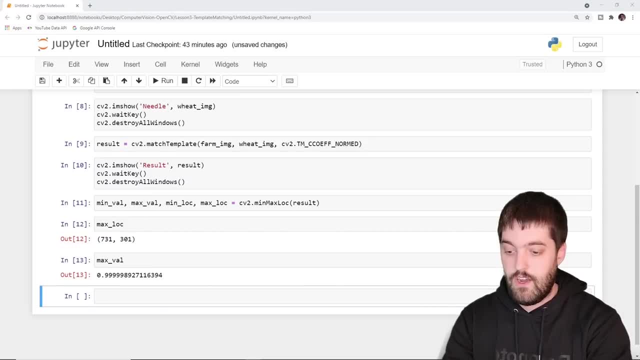 and draw a rectangle around our best match. Now, if you remember, when you're drawing rectangles we need to define a top left point and then a box over the top left point. This way you could draw some lines, that bottom right point. Well, we have our top left point here in our max location. 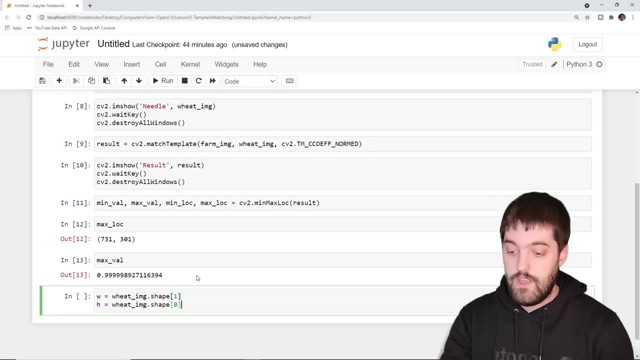 we need to define a bottom right. So one thing I know is how big my wheat needle image was. So I'm gonna get the width of my needle image, the height of my needle image, and then I can add those values to my max location. 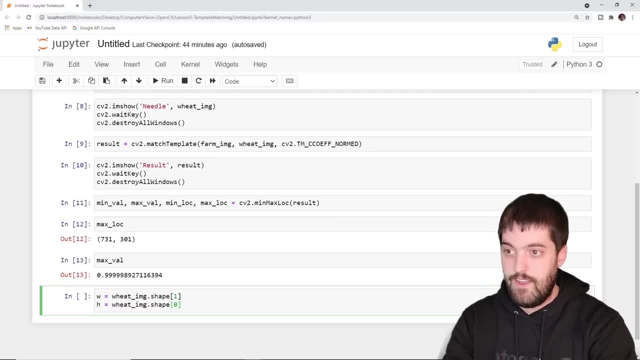 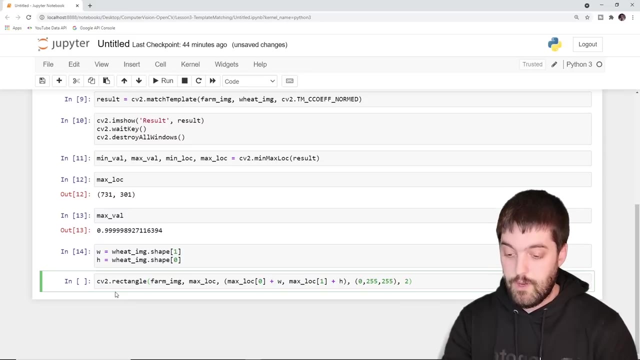 to get the bottom right point on the image. So now that we have the width and the height, let's go ahead and create our rectangle. So to create our rectangle, you might remember we're gonna do cv2.rectangle, we're gonna pass in the image. 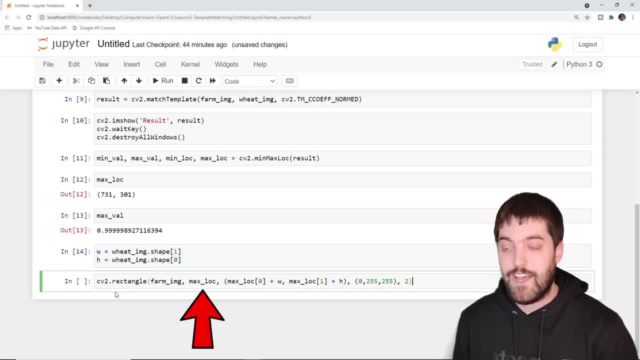 that we want to draw the rectangle on. we're gonna pass in our top left point, which was defined up here in max location, and then we need to define our bottom right point. Now this is a little different, so we're gonna take the x value out of max location. 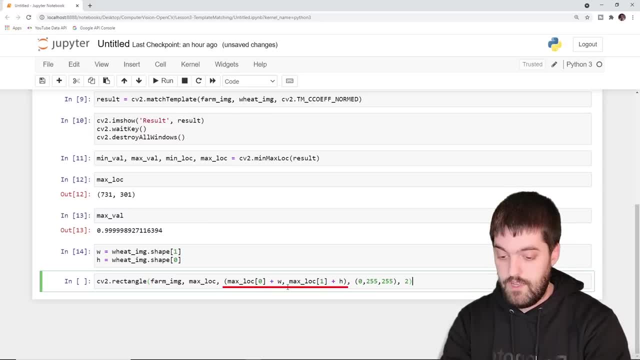 which was in the zero index, and we're gonna add the width to it. Then we're gonna take the max location that was in the one index, which is the y axis, and add the height to it. Then we're gonna draw a box around that. 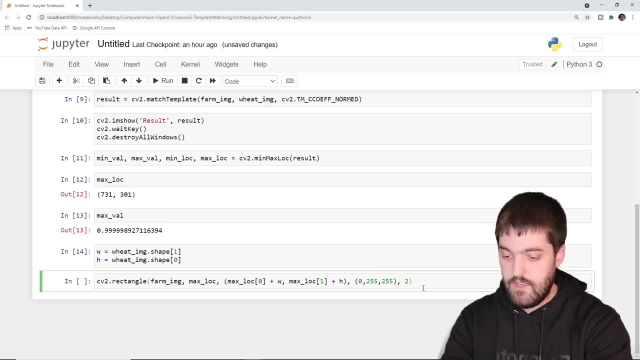 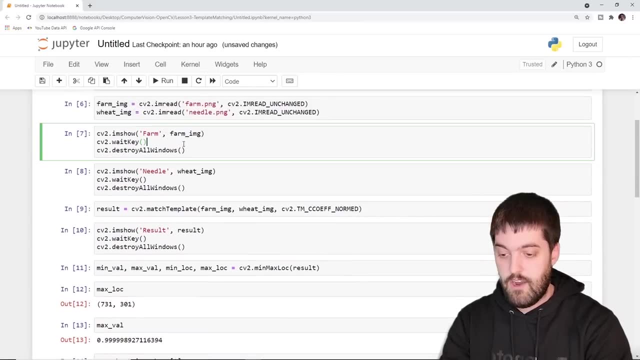 and this is just color and line thickness, if you remember from our last video. Now we can do shift, enter. you'll get some output here and if we go back we can display our farm image again. So I'm gonna go up to the cell that had our farm image. 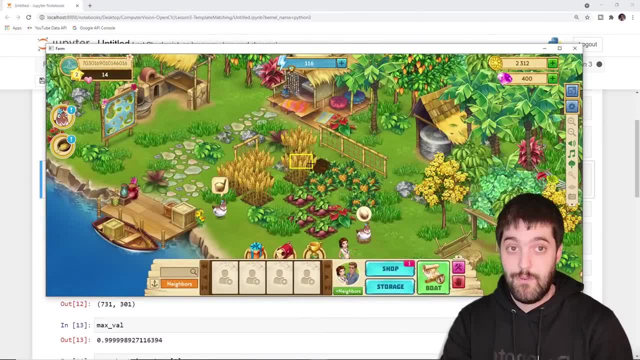 and you can see that our best match was right here, which is probably where I cut the image out of. Now. you're saying: great, we found the exact image. that doesn't do us a lot of good, right? We wanna find similar images. 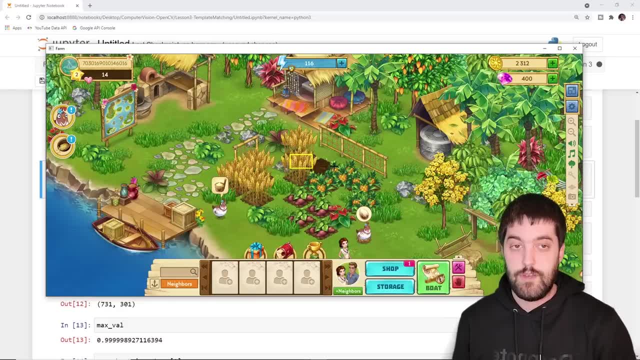 if we're creating a farming game, or if we're saying, do something when you see a mask- it's not gonna be the same mask every time- or something like that. So what we're going to do is we're gonna now define a threshold. 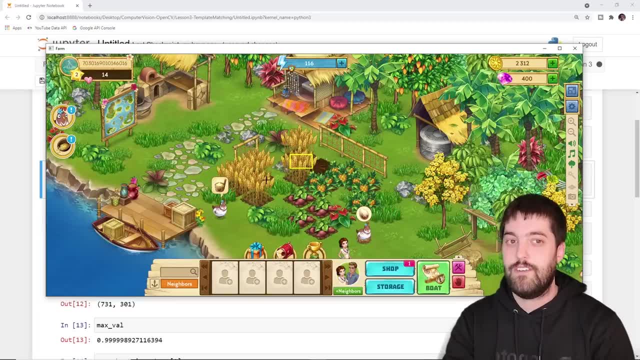 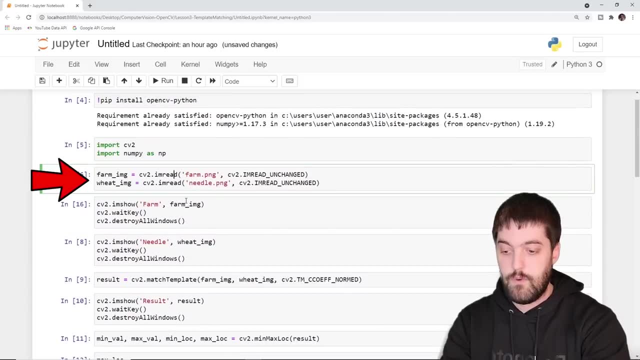 so we can hopefully highlight all the ones that are close enough matches that we think it's wheat. I'm gonna close this now. remember, every time we do something different we wanna reload in our images, so I'm gonna run this cell. 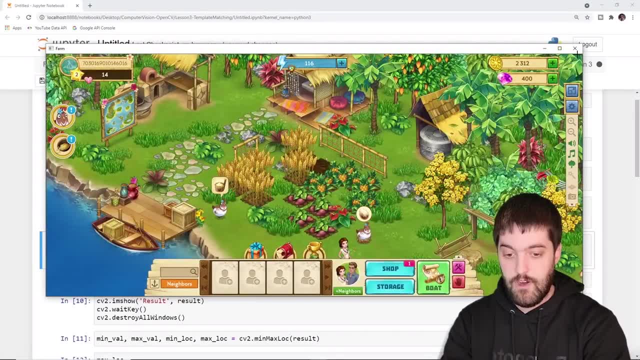 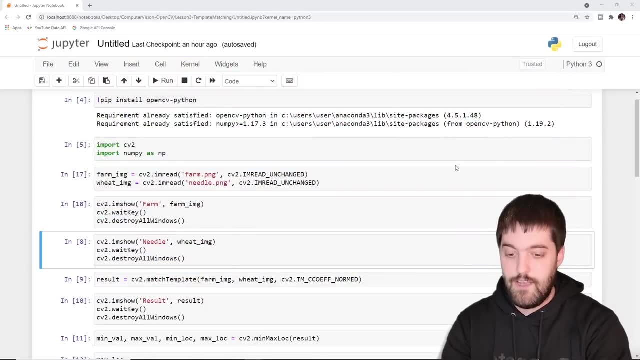 and I'm doing that, so we no longer have our yellow marking on that And now we can go ahead and create our threshold. Now I've done this ahead of time, so I'm just using a threshold that I know works pretty good at finding the different images. 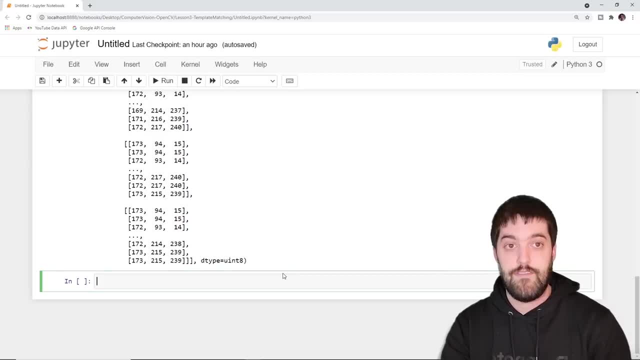 You're gonna have to play around with that. in your example, it might be 85, it might be 60, maybe it's 40. So what you know is if you have too many false positives, you want to try and increase your threshold. 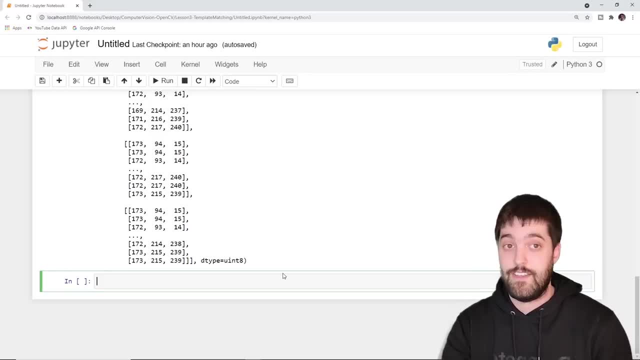 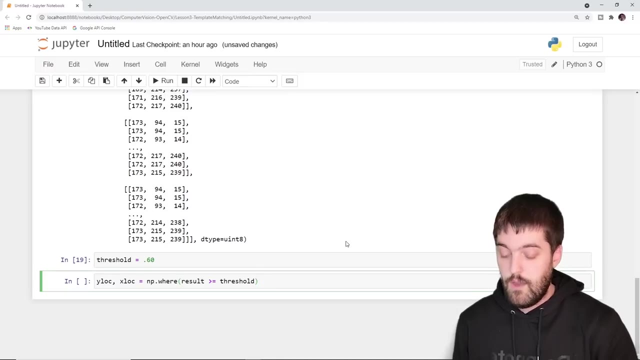 make it harder to find a match. If you don't find all the things you wanna find, you might wanna lower your threshold to find more matches. So what we're gonna do is we're just gonna use a threshold of 60.. Now we can do some NumPy arithmetic here. comparison here: 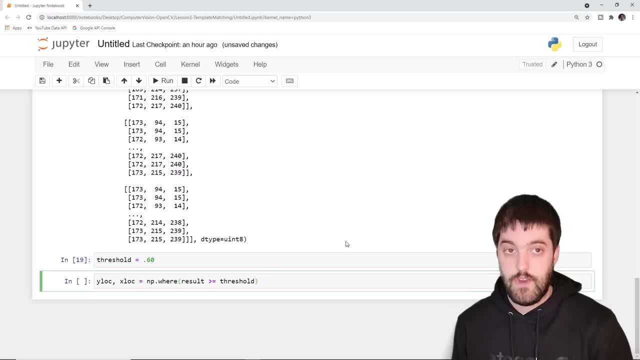 and we're gonna say: where our result is greater than or equal to our threshold, we wanna keep those locations. Now, remember that's gonna return two different results. it's gonna return a Y location and an X location, and then they're in the opposite order you would think. 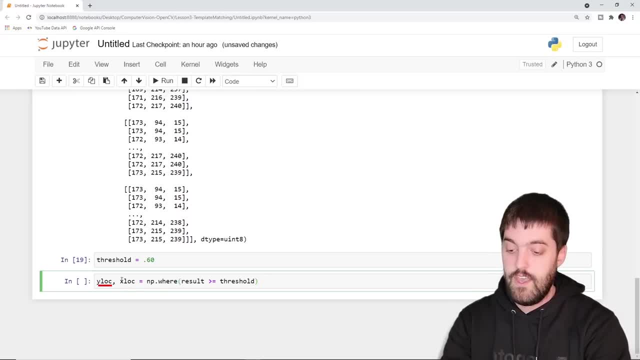 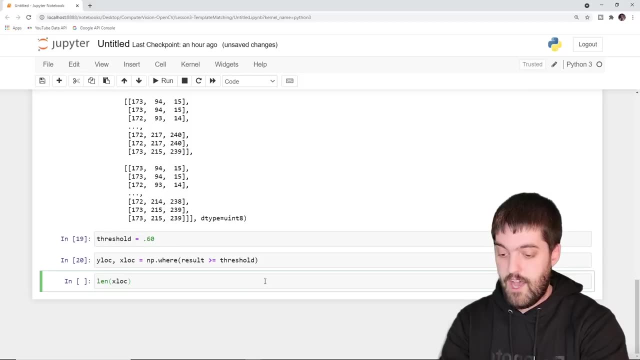 So what we're gonna do is we're gonna receive in some Y locations and we're gonna receive in some X locations here. Now, if we look at one of these, we can see about how many matches we have. So you can see that we got 13 matches here. 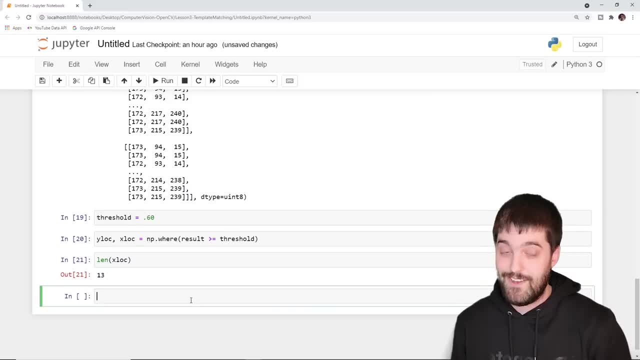 we have 13 X locations and presumably, hopefully, 13 Ys. So now to draw our 13 matches, which you're probably thinking that's too many matches, right? He said this worked pretty good. Hang with me for just a second. 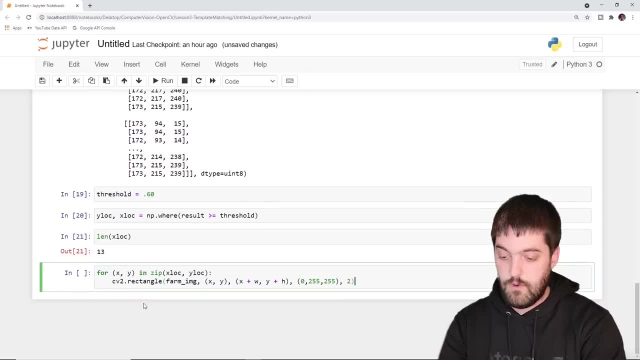 So we're gonna draw our 13 matches. What we're gonna do is we're gonna do a little for loop here. We're gonna do for X and Y. you'll notice I put them in the correct order this time in zip: X location, comma: Y location. 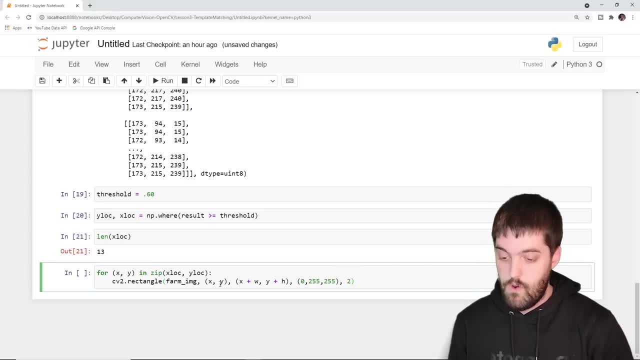 So again, I'm putting them in the correct order- X, Y coordinate- and I'm zipping them together. So I'm pairing each one. So the first item in the X location is paired with the first item in the Y location to create our points. 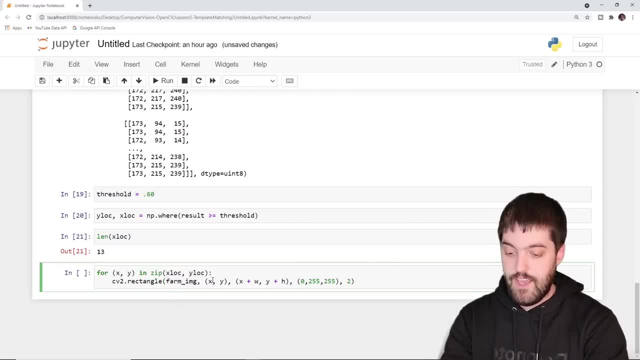 Then each time, through this, I'm drawing a rectangle on the X- Y coordinate. I'm doing just what we did before: On the X coordinate, I'm adding the width. on the Y coordinate, I'm adding the height and then I'm drawing the square. 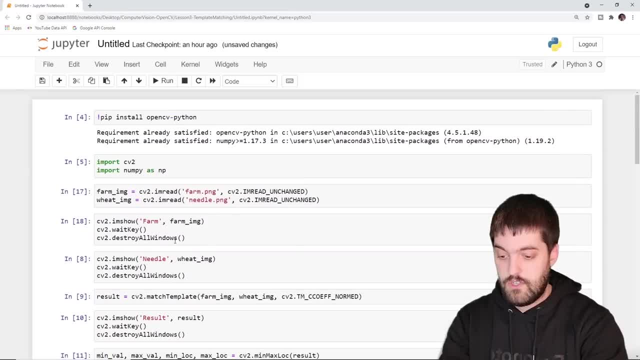 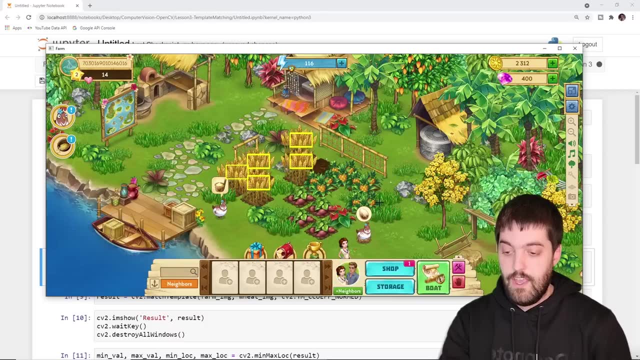 Now, if I run this, I can go back up and I can show our image again And you'll see that we got all five of our wheat images. And you may ask yourself: well, we did get all five, but it said we had 13 matches. 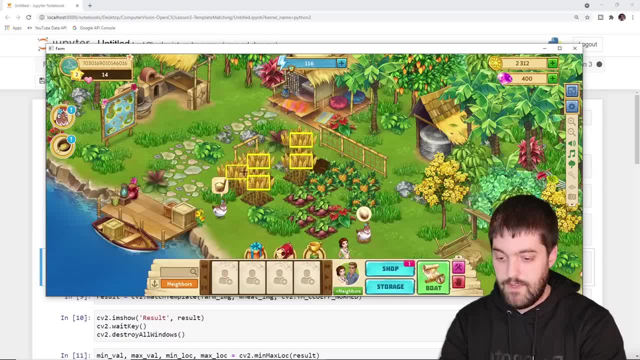 You'll notice, some of these have a thicker square around them than other ones, and that's because it's finding multiple matches. Now, maybe this isn't an issue in your program, or maybe it is, So what we wanna do is show a way. 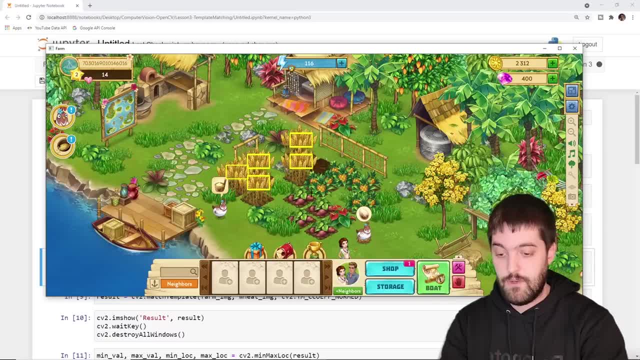 that we can limit it to just the one match. So essentially we want each five to show up, but we don't want multiple highlights over the same patch of wheat and that sort of thing. So we can use another algorithm built into OpenCV. 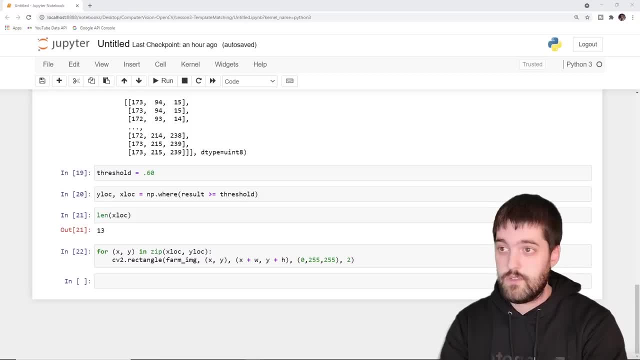 that allows us to group these together. So what we wanna do is we want to create a group of rectangles and then we're gonna use a function that's built in to combine those rectangles if they overlap. So what is a rectangle? Well, in OpenCV, in this algorithm, 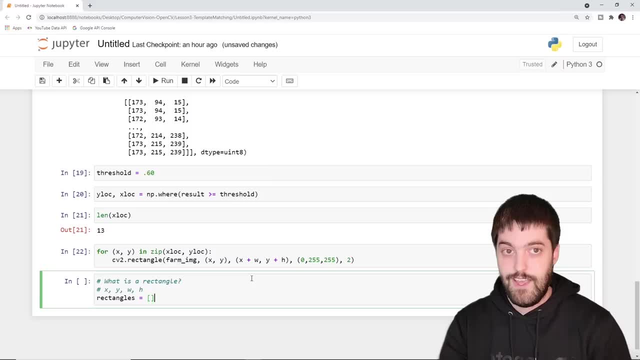 it wants an X coordinate, a Y coordinate, a width and a height for each rectangle, Which is pretty easy. That's basically what we have anyways, So we're gonna create a blank list to hold our rectangles And remember: here we're trying to look at another way. 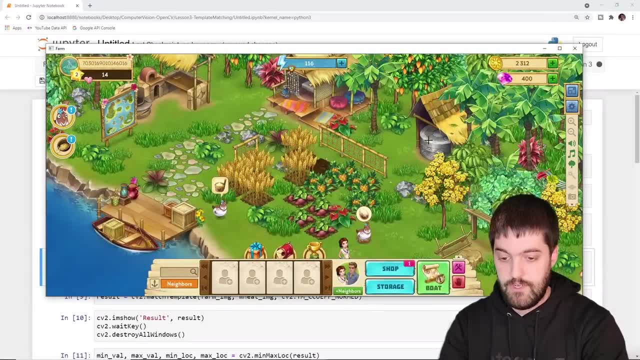 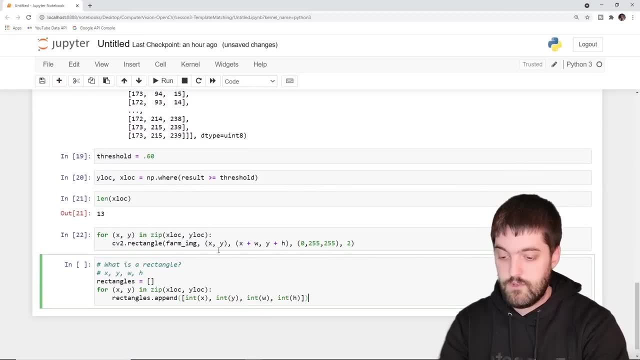 to do this. so I'm gonna reload my images. So you wanna reload that image? so we're back to a clean slate here, And this time, each time through our for loop, instead of drawing the rectangle right away, we're gonna append the rectangle to our rectangles list. 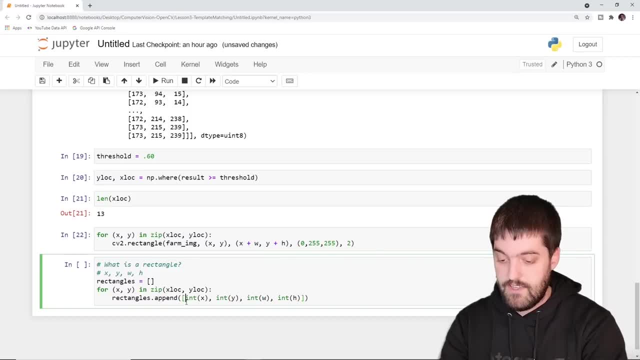 So you'll notice we're doing rectanglesappend each time and inside of this we're using square brackets. so it's a list inside of a list And we're defining it just like OpenCV: once X, Y width and then height. 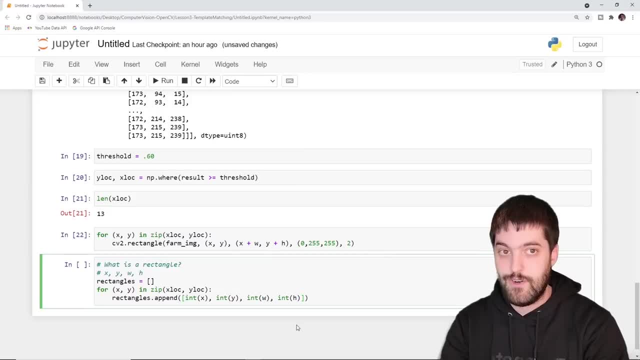 And each one I'm converting to an integer to make sure we're not gonna blow up this function down the road. Now, one other thing you'll notice is: in our case, not every rectangle was duplicated. One had just a single square over it. 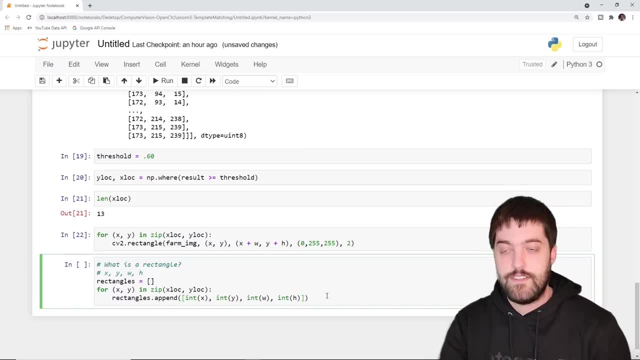 That's gonna be an issue. When the group falls, it's gonna fall, it's gonna fall, and when the group function runs, it's gonna want at least two rectangles to group them together, and that's not the effect we want. 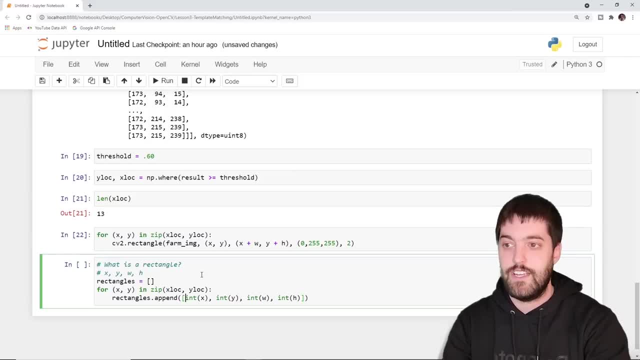 We want it to find all five, even if a single rectangle is over it. Now I've looked at the code and I've looked at a couple other forms and there's basically one workaround to do this and that's to duplicate the rectangles. 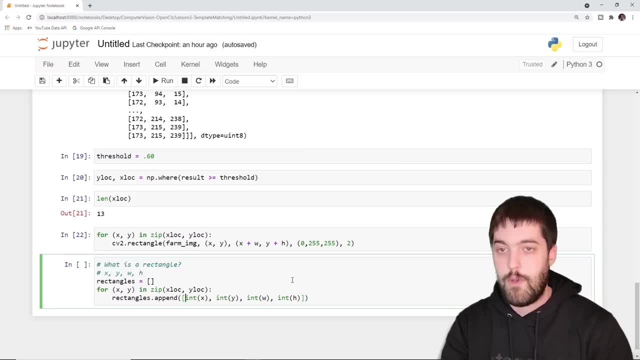 So we're gonna make sure that it has at least two on it by putting every rectangle in there twice. So we're literally gonna copy this line, paste it below and that will duplicate the rectangles as it puts them into our rectangle list. So if we run this, then we can run length of rectangles. 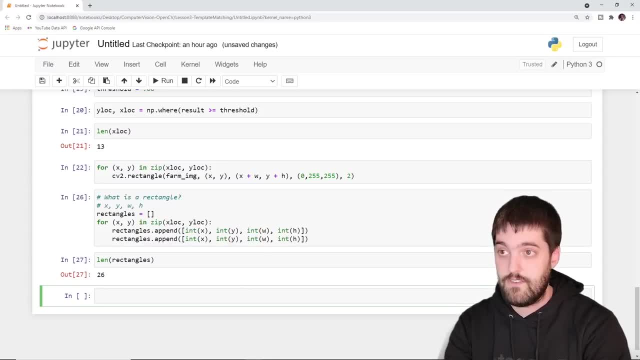 and you can see that we got 26,, which makes sense because we did duplicate those. Now we can pass it into our grouping function. So I'm gonna grab a couple values out here and you can read up in the documentation on these actual parameters. 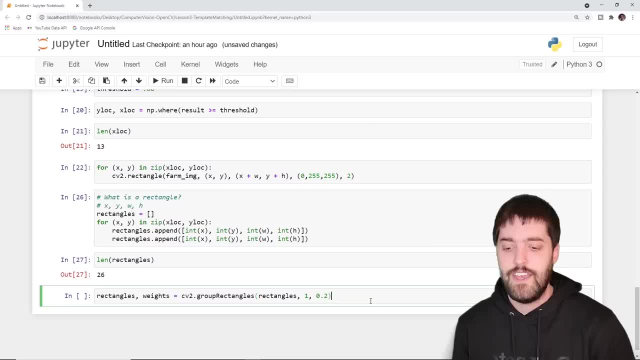 and play around with it to meet your match. So basically, what we're saying here is: how many rectangles do we want in a group? We want just one. So it's gonna pair those down and then there's a coefficient here that you can play around with. 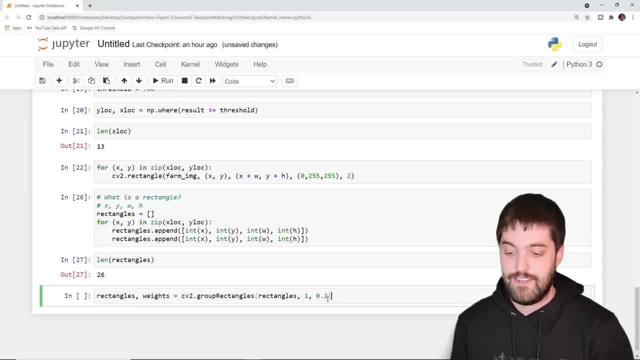 It'll basically say how close it has to be to consider it a group. So how much of an overlap is okay to group them together? This is the parameter that I found was useful. Go to the docs right here and you can play around with these values as well. 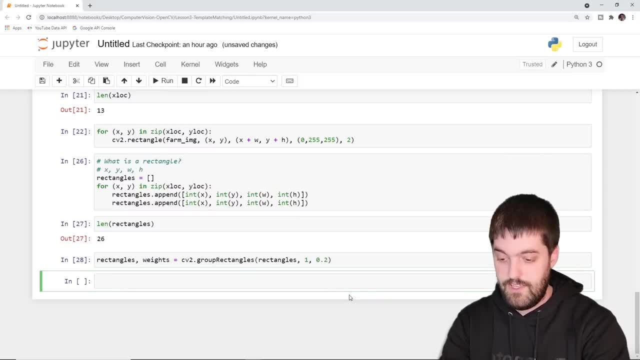 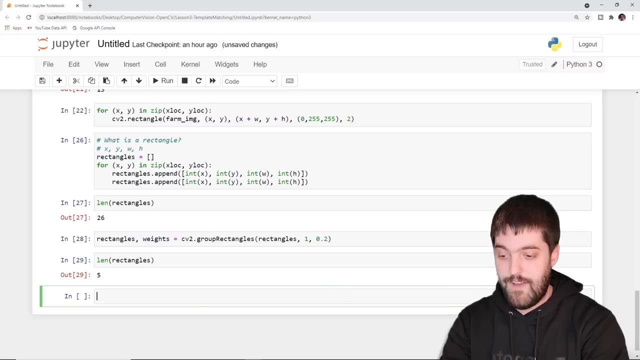 in your own problems. So we're gonna go ahead and run this, And now we can take a look at the length of our rectangles again and you can see that we're down to our five, which is very promising. Now let's copy our function from above. 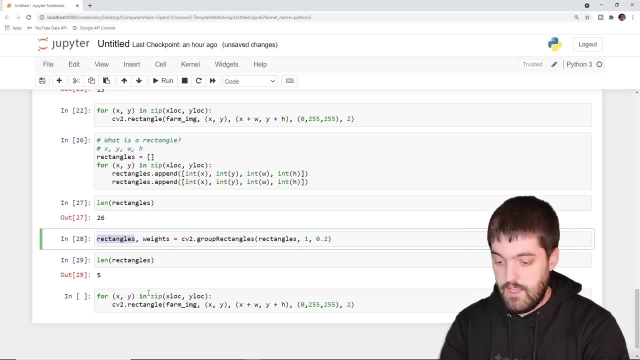 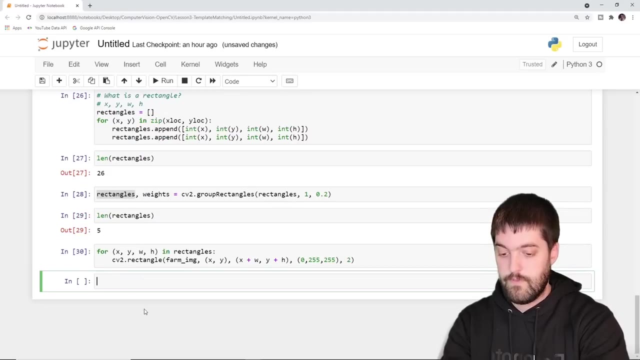 our for loop that drew the rectangles And instead of iterating over our zip, this time we're gonna iterate over rectangles and we're gonna unpack from rectangles each time an x, a, y, a width and a height. Now we can run this. 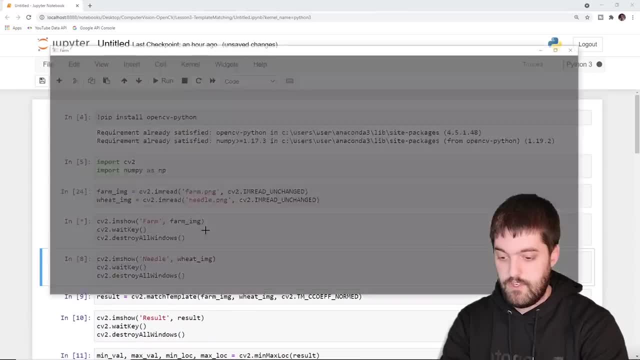 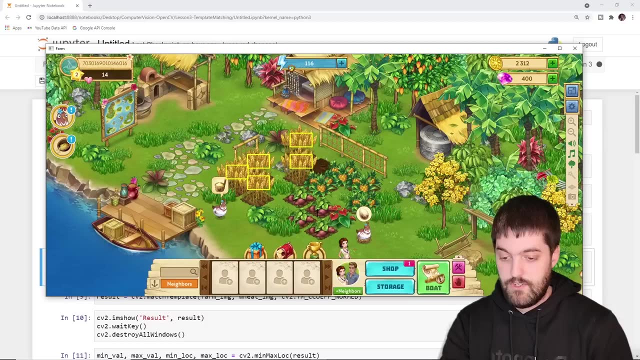 Let's slide up and look at our farm image And you can see perfect. we got five exact matches that look perfect for our image, so that's exactly what we wanted. Now, this is a very simplistic example, but it gets you started and shows you exactly how to do template matching. 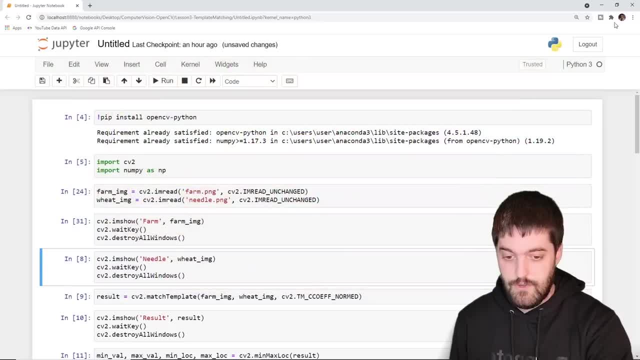 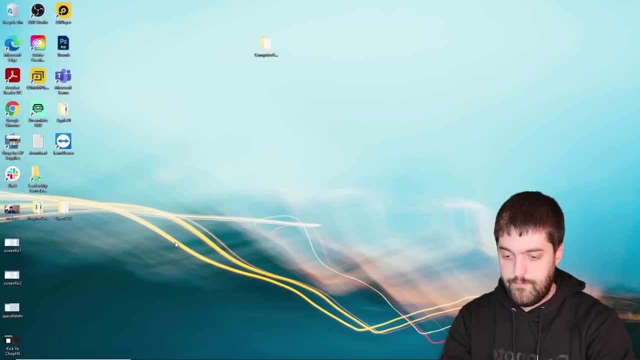 Now I wanted to do a fun little program just to highlight this even more. So what we're gonna do here is we're gonna take a look at another example. look, I'm gonna do this. look example of template matching really quick here. so I don't know about you. 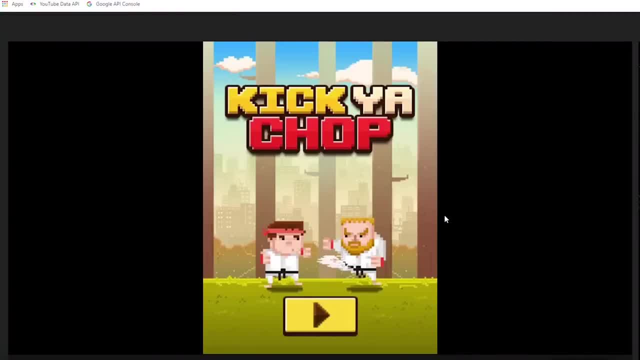 guys, but in my childhood I like to play a lot of these silly flash games. now they're mostly HTML 5, but we're gonna use that to show another example of template matching here. this is called kick you chop, so the concept of this game is really simple. if you click on the left side, you break a branch off of. 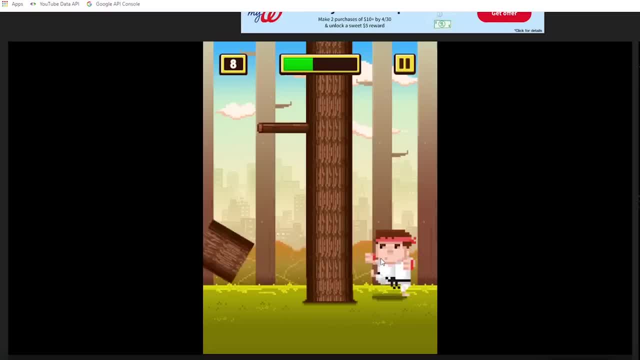 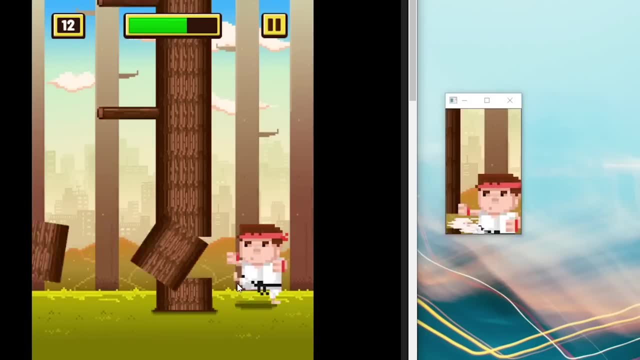 the left side and your guy stays on the left side. if you click on the right side, he moves to the right side and you need to avoid the tree branches that come down. I'm gonna show you my best run here, or one of my best runs on my way to. 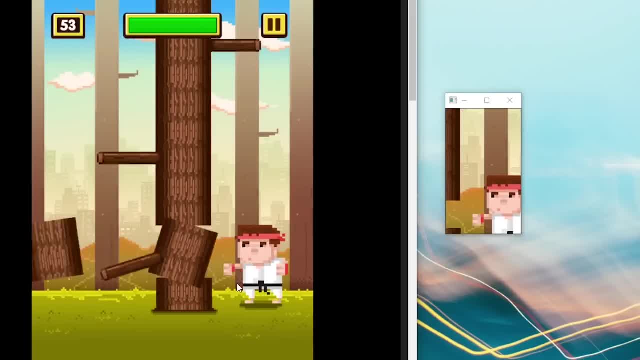 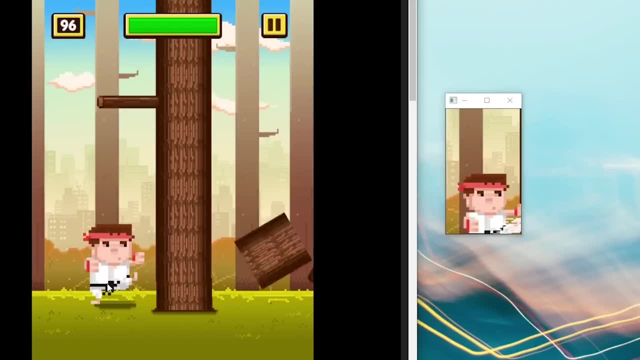 getting the highest score and kick you chop. the program is really simple. it's just gonna test using template matching to see if there's a branch above our man's head, and if it is, we're gonna click the opposite side. you can see here that it's testing above the 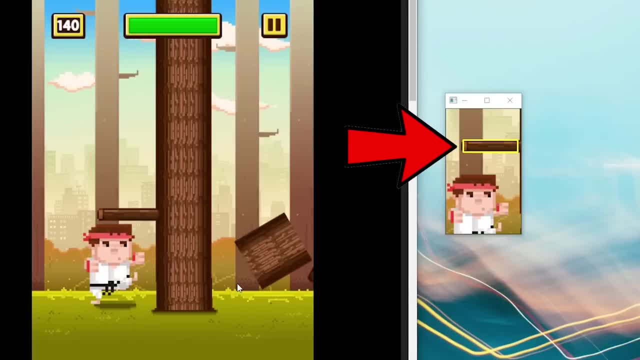 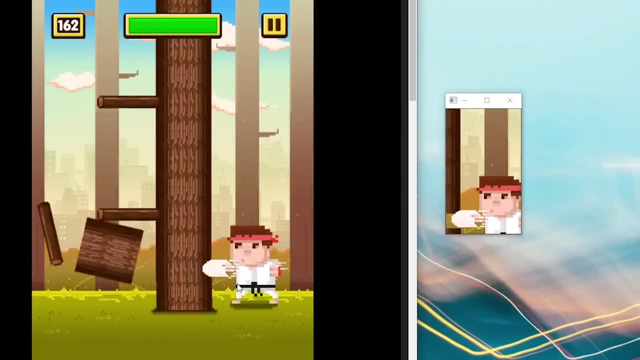 player's head to see if there's a branch there, and when there is, it's clicking on the other side. so I'm doing this using screenshots with MSS and then pie auto GUI to actually click the screen either on the left or the right. you'll see the 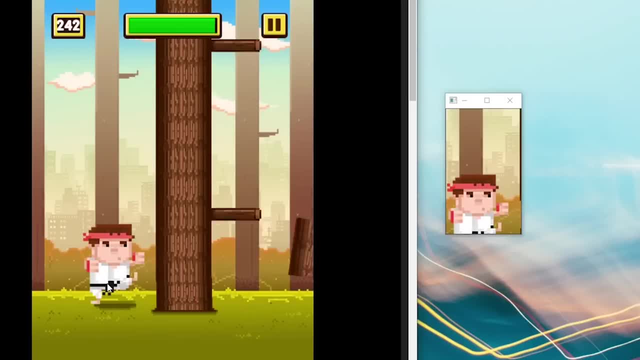 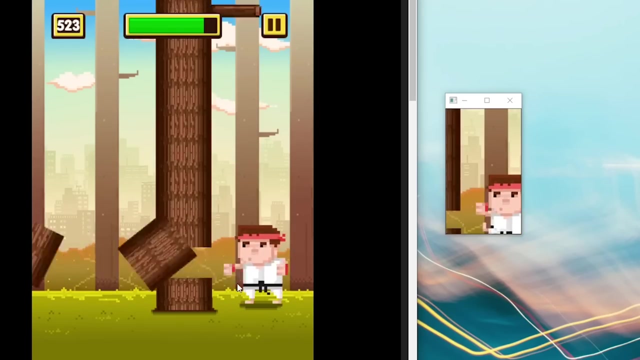 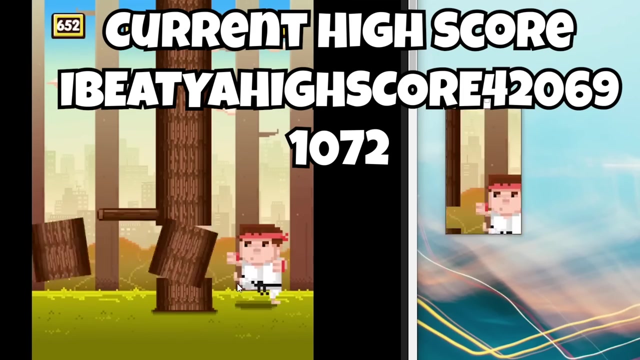 mouse moves on its own. now I simply took a section above the player to test, so I needed to use a stick from the left side and a stick from the right side as my needle images. if I'm on the left side of the screen, if my players on the left side of the screen, I use 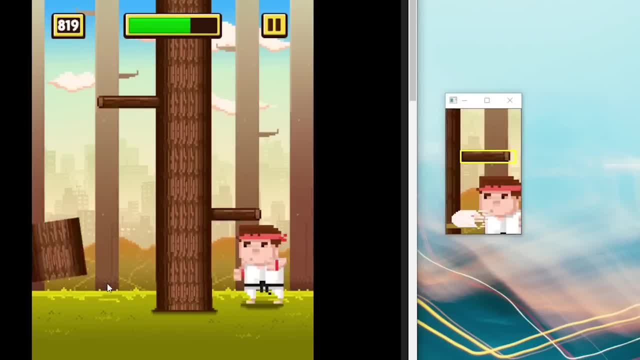 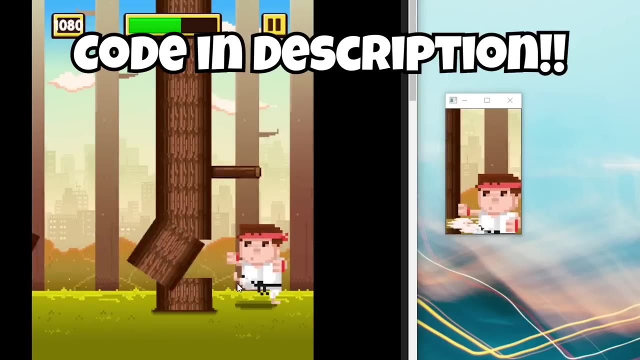 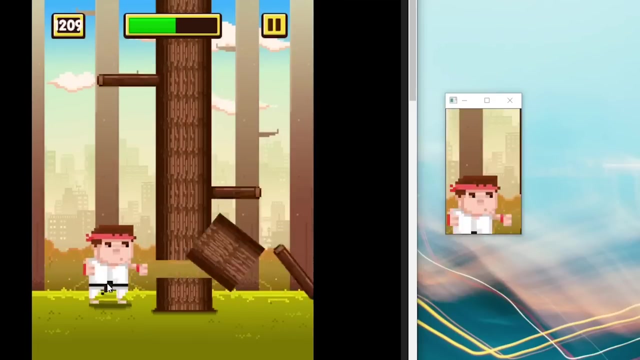 the left image if my players on the right side of the screen. I use the right image and I only test whichever side I'm on, because that's the only time I'm worried about a branch hitting me in the head. now, if you run out of time with the green bar on the top, you lose and also